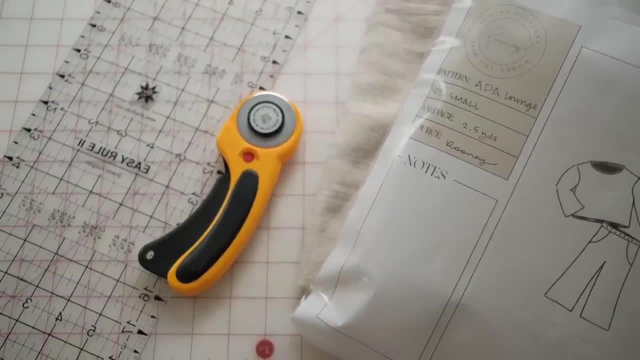 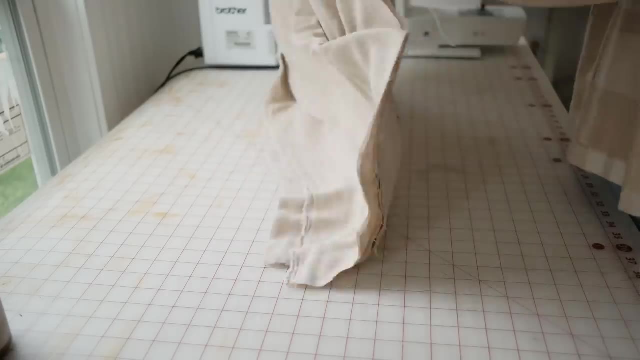 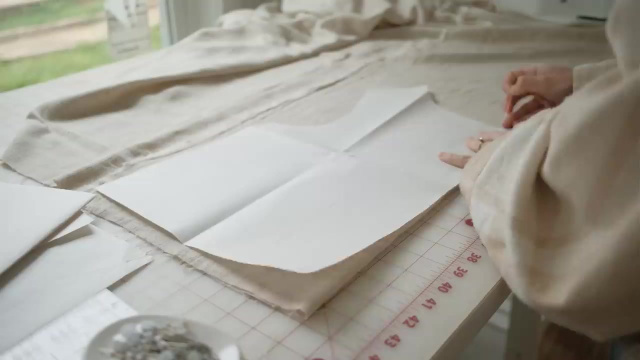 what I like to be comfortable in and really just take the time every day to make something and enjoy the process of putting the spring wardrobe together. The irony is it's cold and rainy, but it has been fun to have this space and even throughout the cold and the rain, look forward. 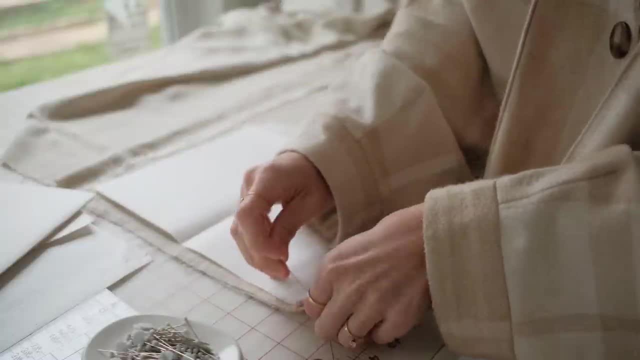 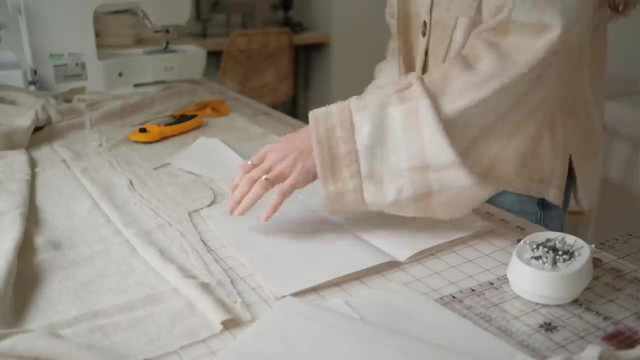 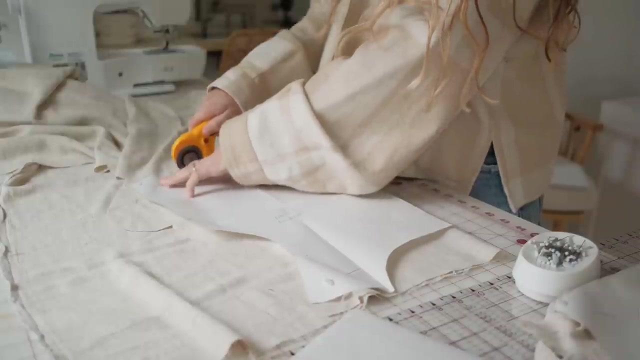 to the warmer weather, the blooming of the flowers that I'm already seeing spring up and the vibrant colors coming out through nature, And I think the juxtaposition of the weather and what I'm looking forward to is a really good reflection of life and makes me just really grateful to be able to. 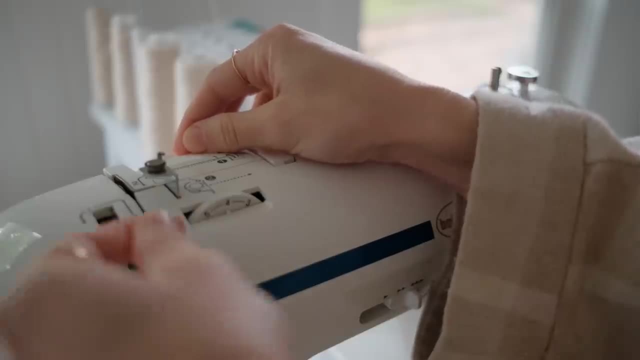 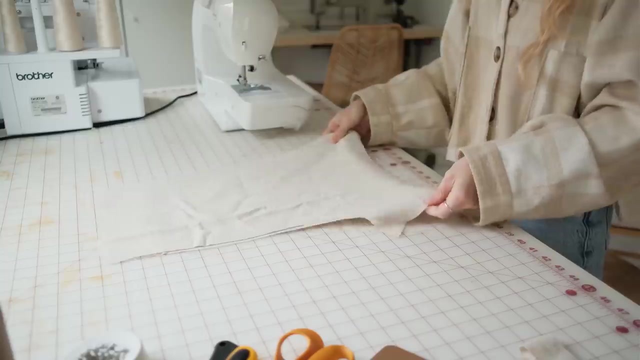 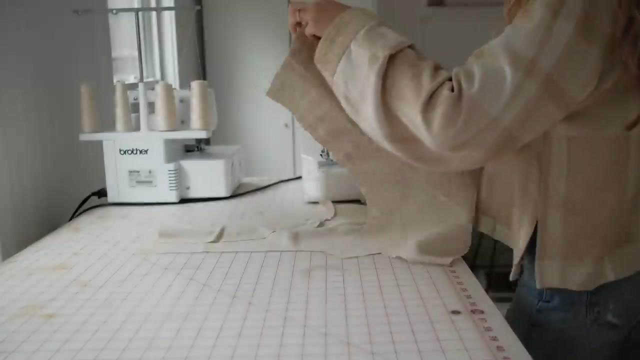 enjoy the process while looking forward to the future. I wanted to ask you and hear your thoughts on sewing for yourself, if it's intimidating to you or if it's a place of respite. I know that I've heard from a lot of you that sewing for yourself is intimidating and I wanted to hear more about. 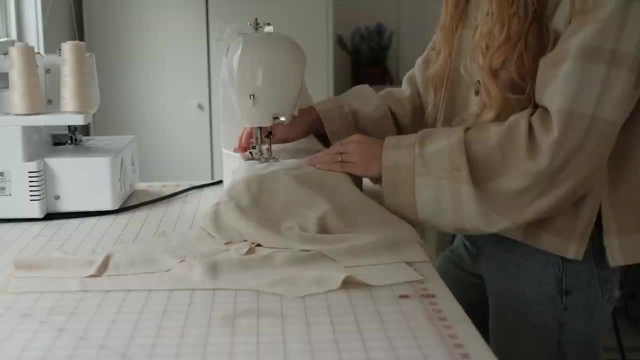 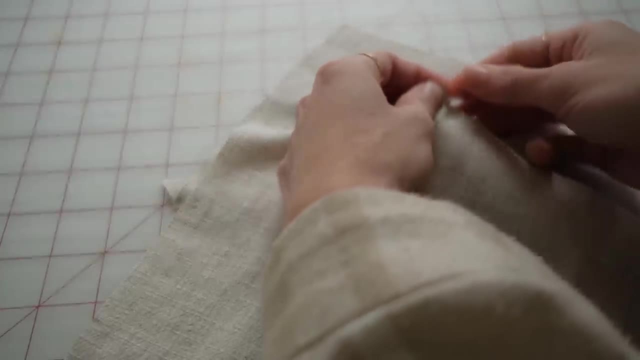 that. I think that sewing for an adult, and especially if it's something you're sewing for yourself, is really enjoyable and can teach you a lot about sewing, because you can sew and then try it on and kind of see what you want to tweak. I think that's a really good point. I think it's. 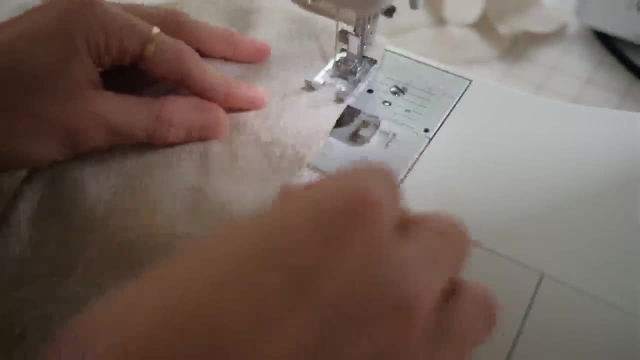 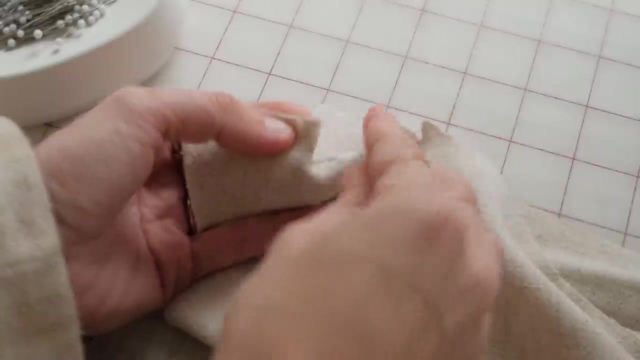 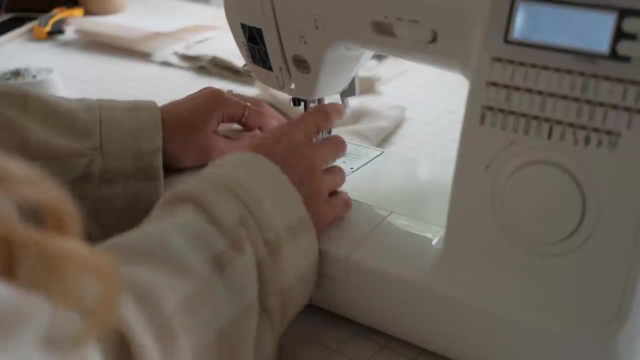 a really good place to start and change where you may want to add length or where you want to make something shorter. So if you like to sew for yourself or if you haven't dove in yet, I would love to hear about that. This video is just a compilation of some things that I've made and 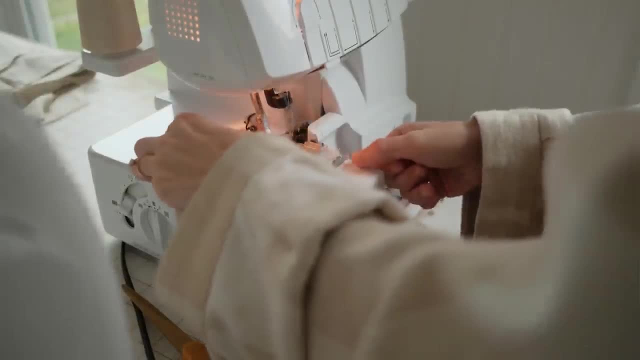 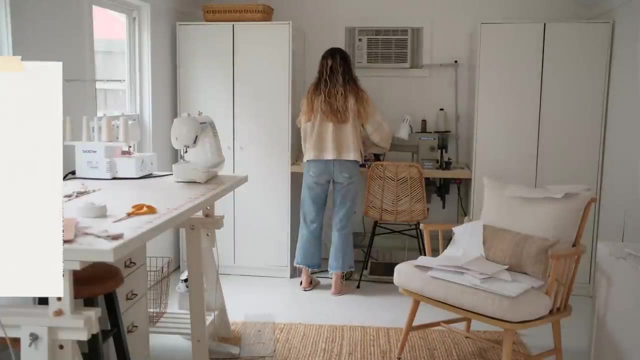 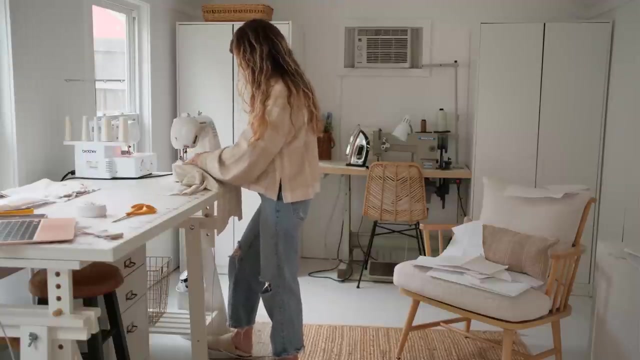 right now I'm making the Ada Lounge set in this linen blend that I found at Joann And I'm making it in two shorts so that I can wear it throughout the summer to farmer's markets, To the beach- hopefully we'll get to go- And just the warmer days where you need a lighter. 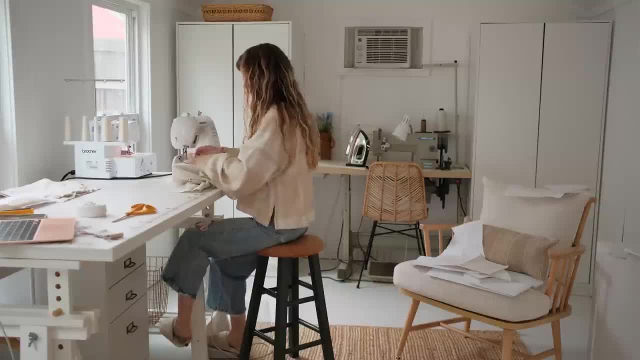 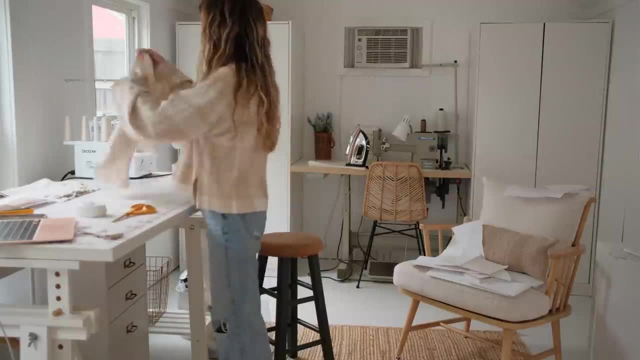 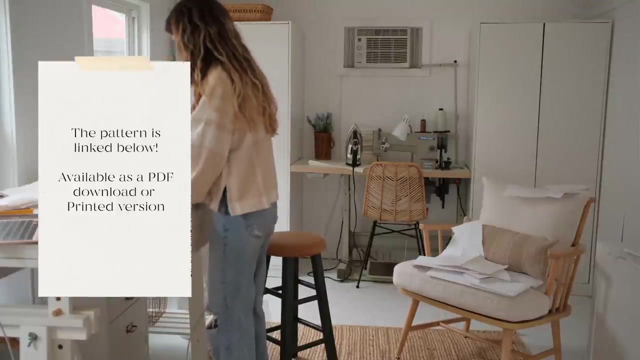 layer and something that feels put together but is super easy to wear. That's why I love the Ada Lounge set. I think it's a great pattern to follow if you're just getting into sewing and you want to kind of branch into an item of clothing that you've never done before. I love the pockets on 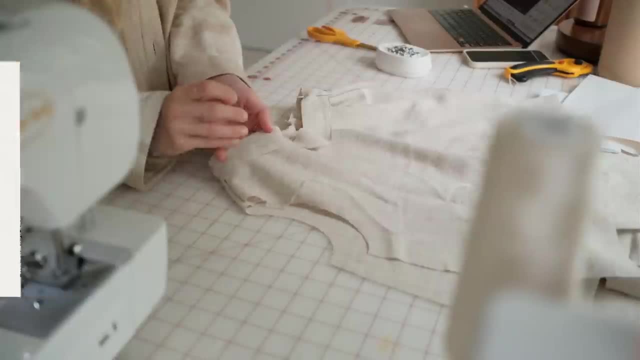 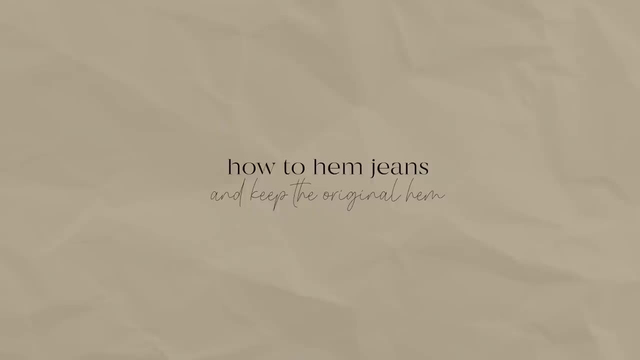 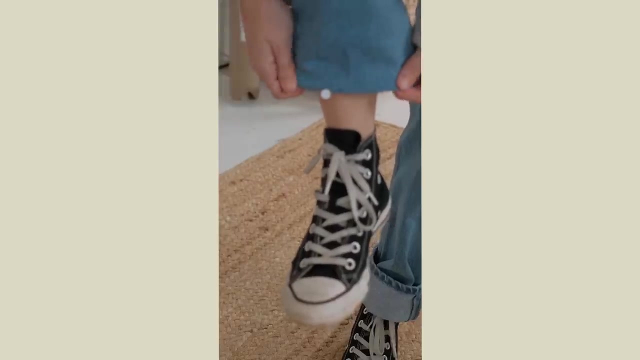 the shorts and the fit of the shirt is really fun too. So I don't make all of my clothes in a set, but I do try to make sure that the clothes that I have fit well and are comfortable. So I found these jeans and I really love the fit of them, but they're a little too long, which is a 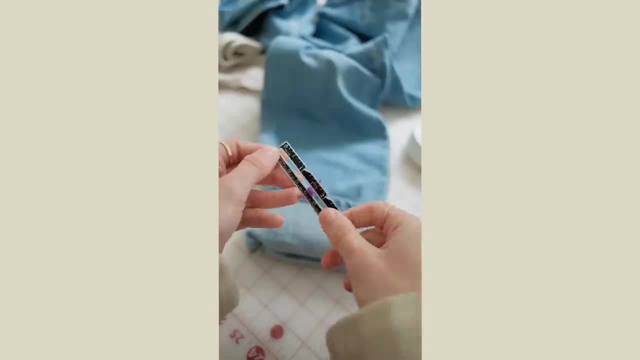 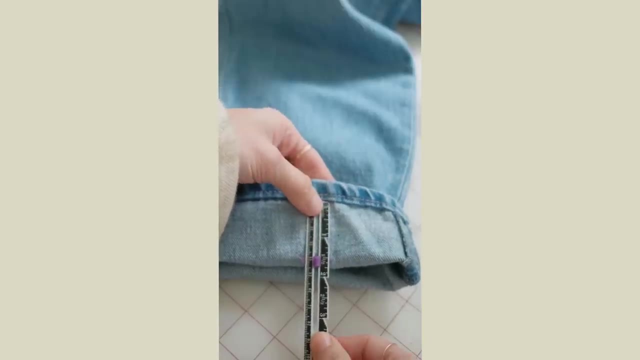 common problem for me, since I'm a little shorter, So I hemmed them, and if you're wanting to hem jeans with the original hem, this is a great way to do it. First, you want to try on your jeans and mark with a pin where you want the bottom of the jeans to be. Then 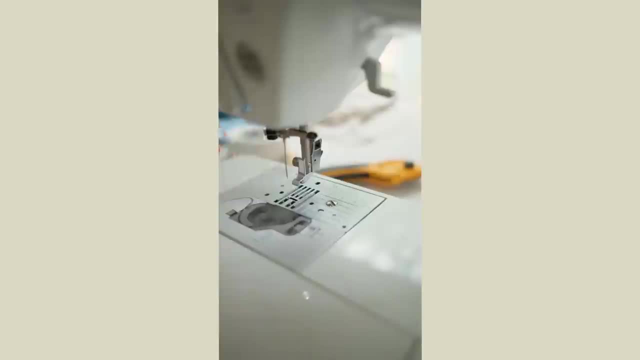 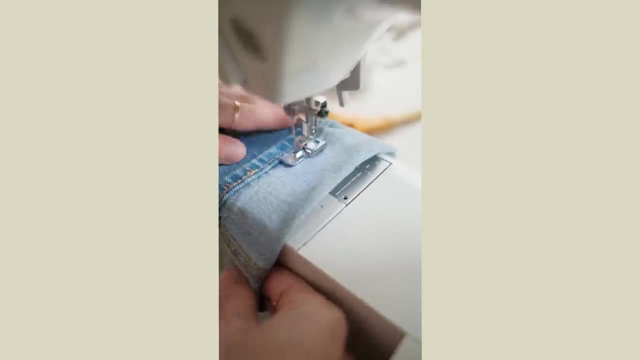 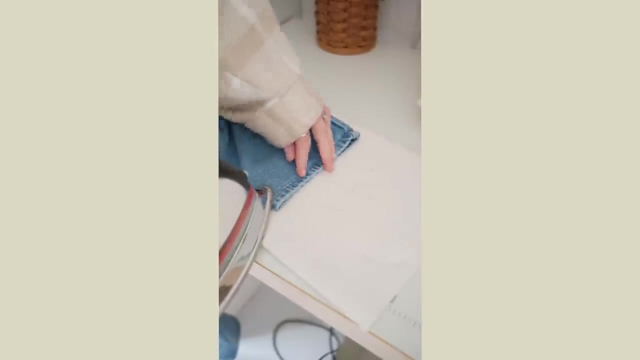 divide this number in half and measure the cuff from the finished hem to the edge of the jeans Using a zipper foot on your machine or you can also hand stitch this stitch along the edge of the finished hem. Turn this right side out and iron- You can give it a top. 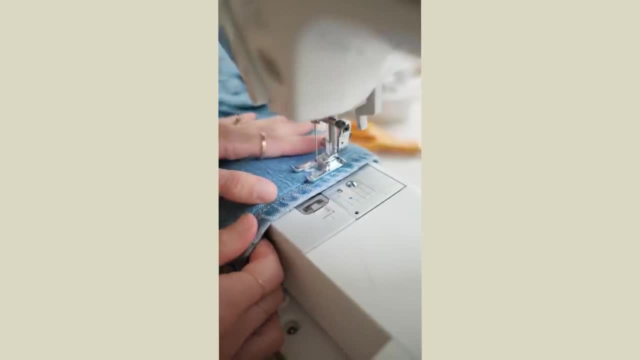 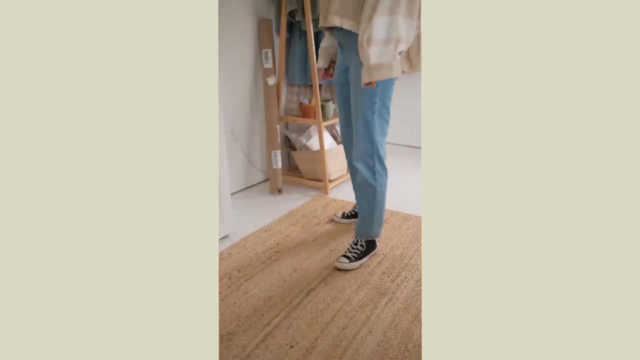 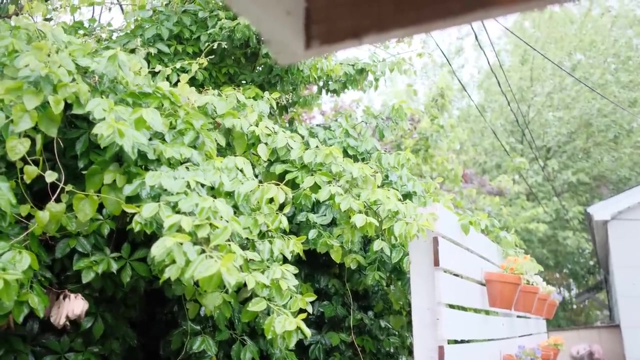 stitch with some coordinating thread, and you can also remove the interior bulk by trimming it down with scissors and serging along the edge or zigzag stitch. Like I said earlier, it has been dark and rainy, and so I'm finishing up the Ada Lounge set today. 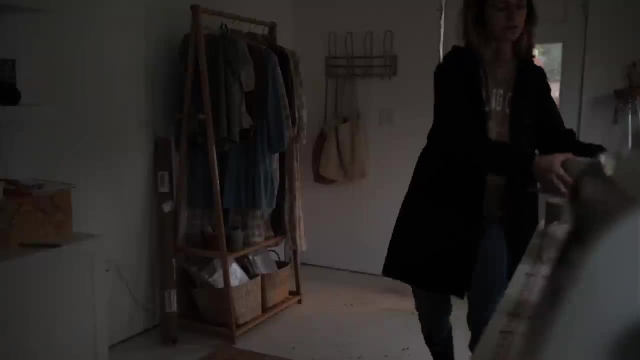 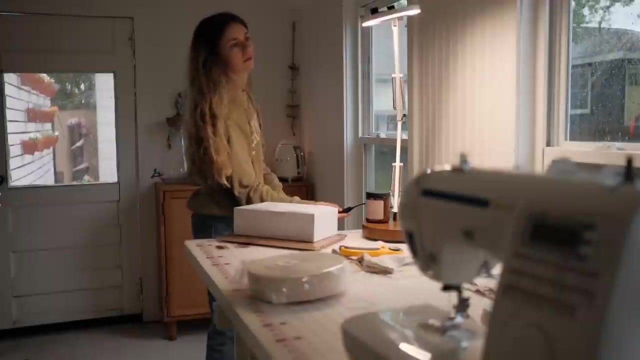 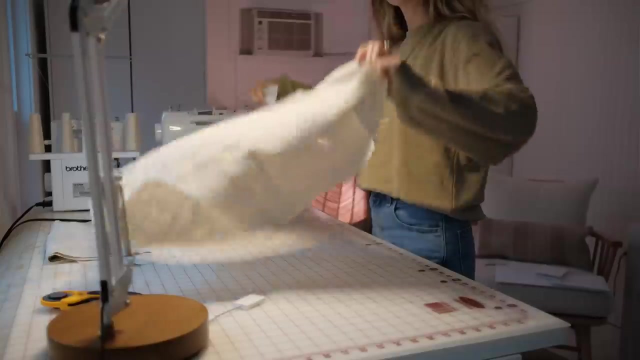 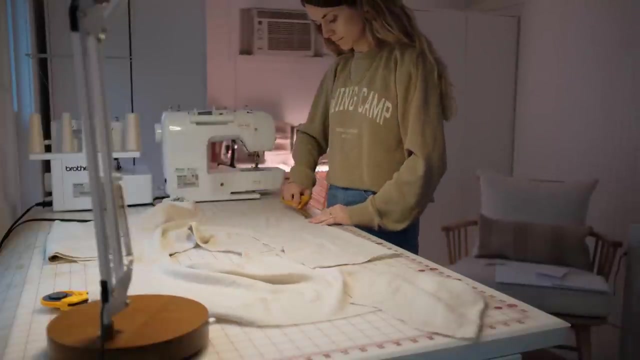 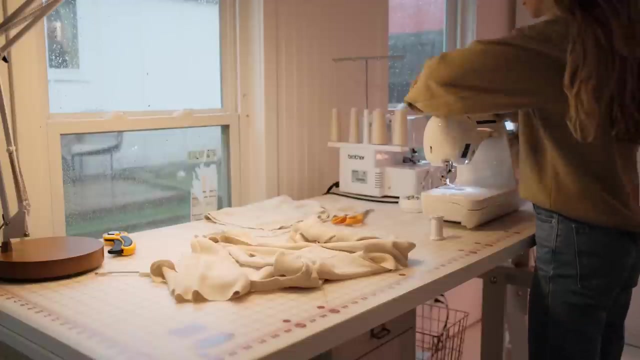 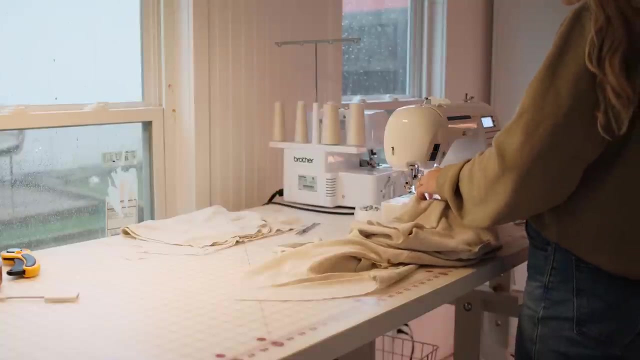 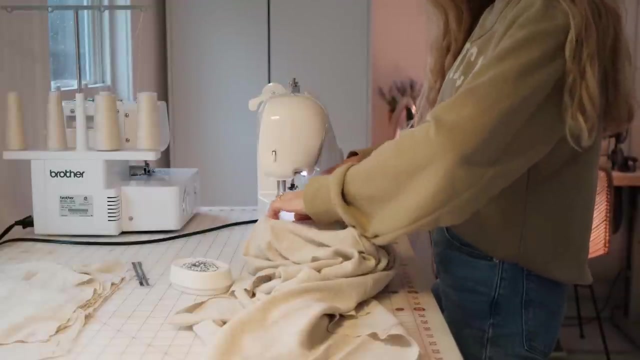 and it has been enjoyable to be inspired by the moodiness that comes with the rain. but I'm not gonna lie: I am excited for this warmer weather. Taking a look at the photos of the house, You can also take two pictures of the house, like this way. Open up the photo and guess what? you took: A photo of a five-star house. Look at this. It's so beautiful. It's the most beautiful. Look at the video. It's so beautiful. We have a lot to share this summer. We have a lot to share this summer. We have a lot to share this summer. We have a lot to share this year, And the summer time is the end And the end of your trip has gone over you. We will be back here. We will be back here again. We will be back here. 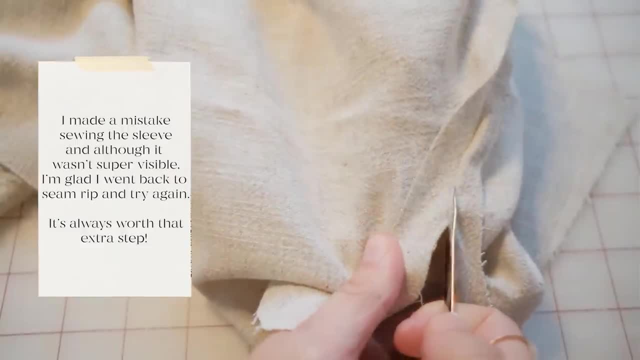 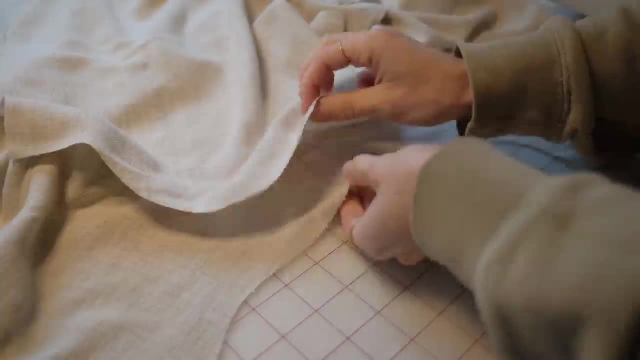 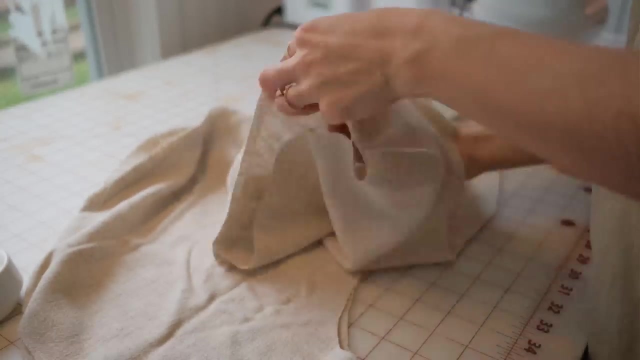 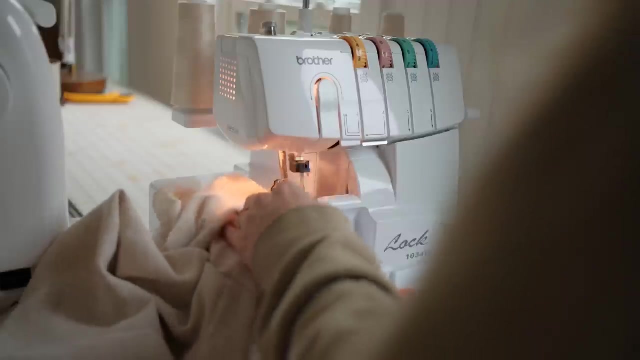 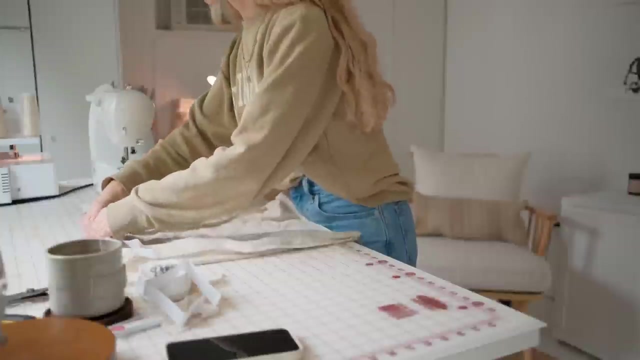 50g unsalted butter. Stir until well combined. Cumin powder: 2 tsp. Baking soda: 1 tsp. 1 tbsp Salt, Sour cream: 2 tbsp. After the hair is dyed, cut the hair in a straight line. This is the most important part: the end of the hair. 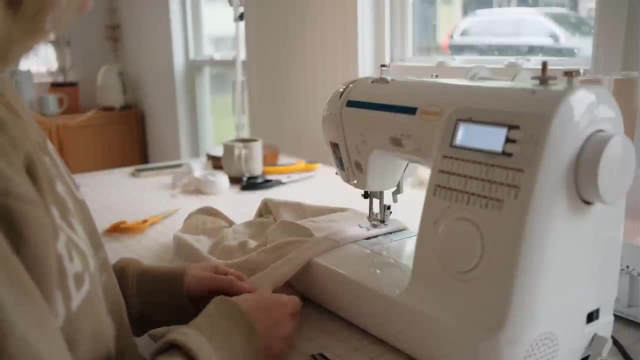 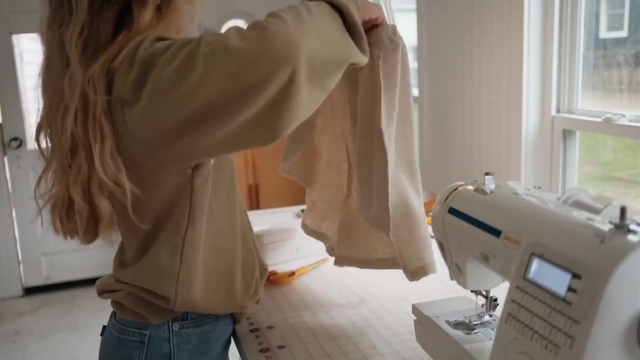 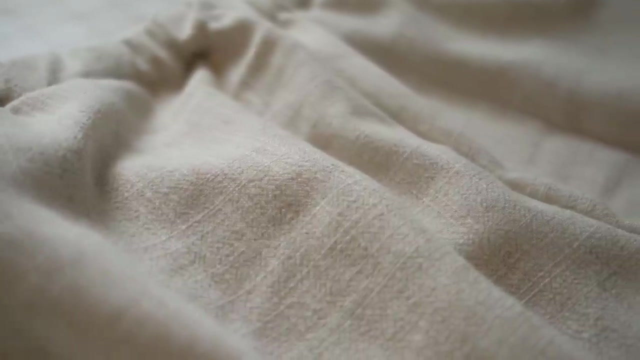 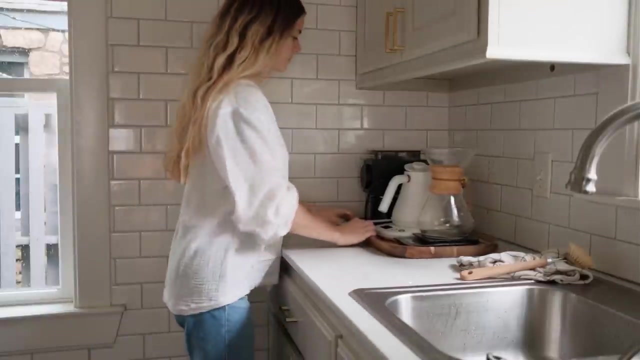 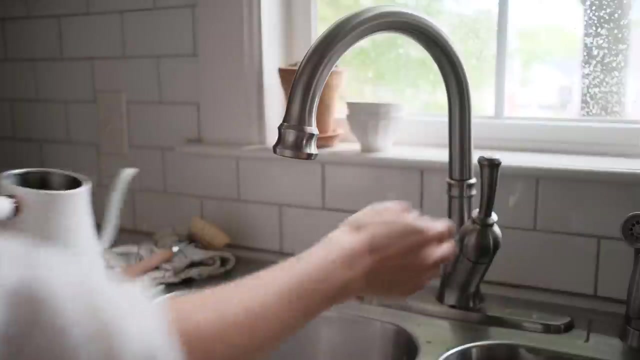 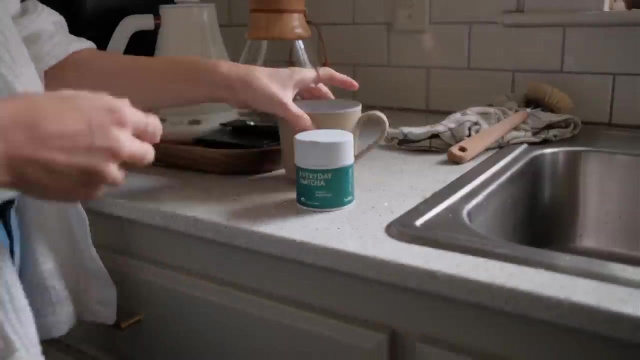 This is the last part of the hair. This is the end of the hair. I will tie my hair with a hair tie. another day of rain reminds me that setting the tone and atmosphere of wherever i'm sewing before i begin sewing is so important to me, and i feel like it makes a huge difference. 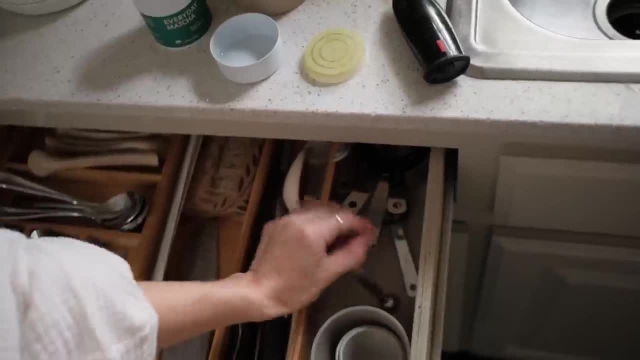 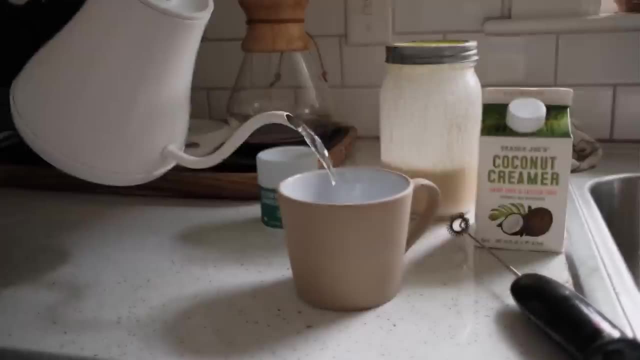 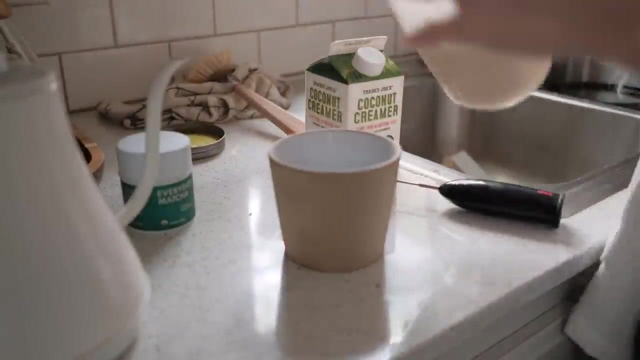 i'm the type of person that just really cares about the atmosphere, especially if it's like at a restaurant or my house. i feel like setting this tone can change my mood. it can change my outlook and give me inspiration of what i'm working on, so that's why i love the process. 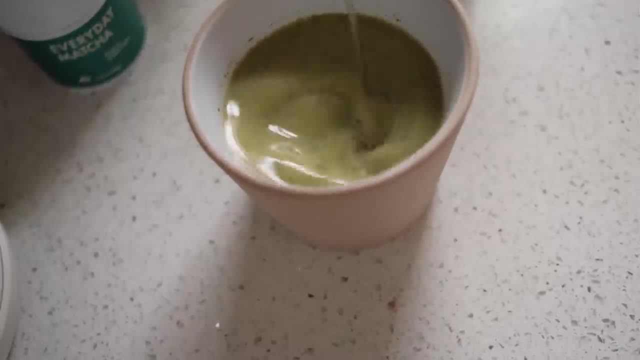 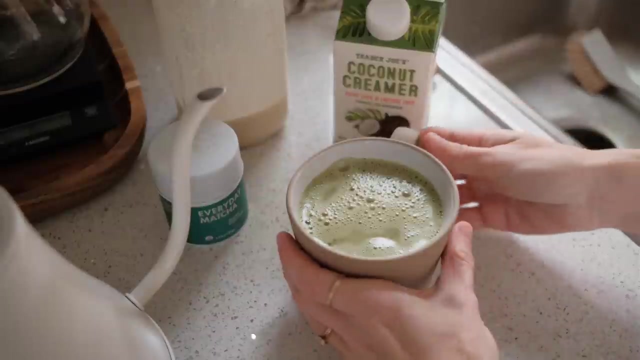 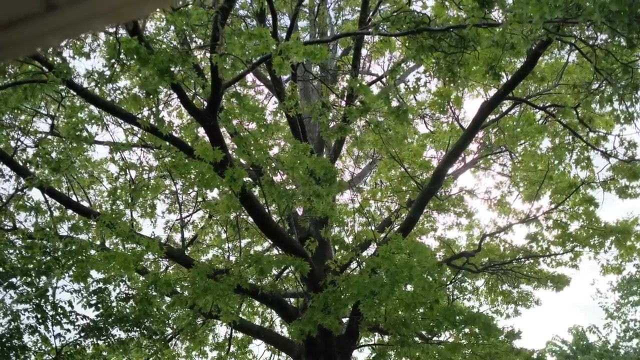 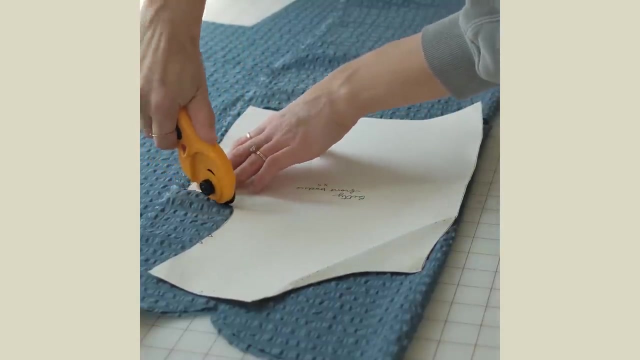 of making tea and i love candles and diffusers and lighting. i think all of the these things just play a factor into the process and to slowing down and easing your mind and getting focused. i made this betty dress out of this silky seersucker fabric from joanne and i. 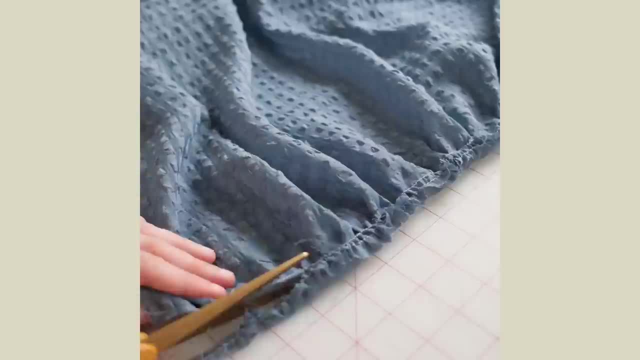 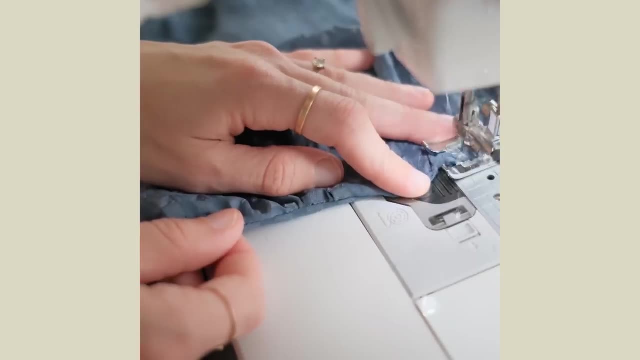 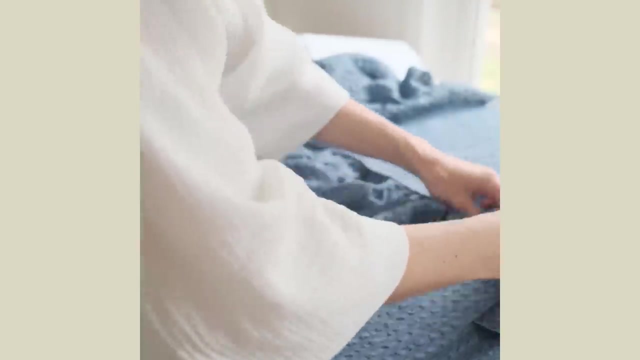 love how light the fabric is, which is perfect for the spring and the summer, and i sewed this using french seams and i think it just took this up a notch and since the fabric is a little see-through, i think having those french seams really made a difference in the end product.